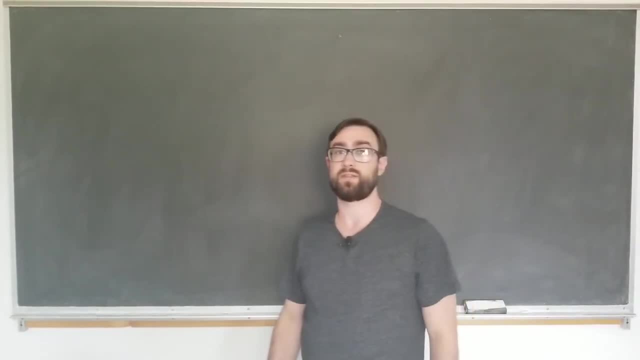 Hi everyone, welcome to Mostly Math. Today I'm going to show you some useful tips and tricks to evaluate trigonometric identities using complex numbers. So you might come across instances like this in an exam: Sine 2x, What's that? I don't remember the formula. Or how about cosine squared? 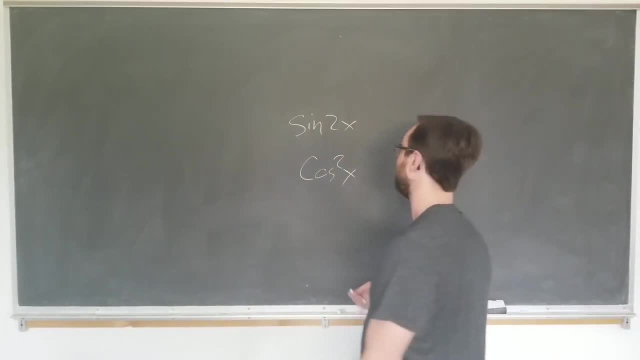 x. What's that? I don't remember the formula for that either. And how about sine of x plus y? I don't remember. There are two formulas and your instructor just hasn't given you a formula sheet and you had to derive them. How would you do it? Easiest way is the way that I'm going to show you. 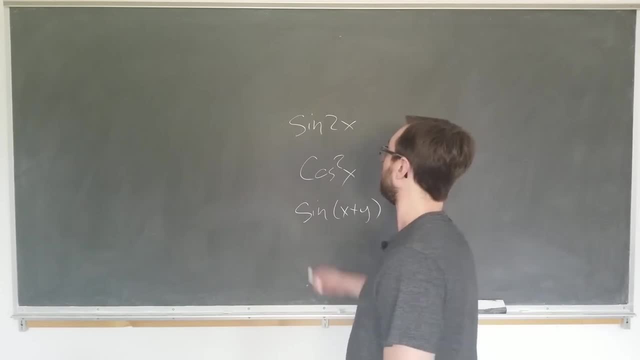 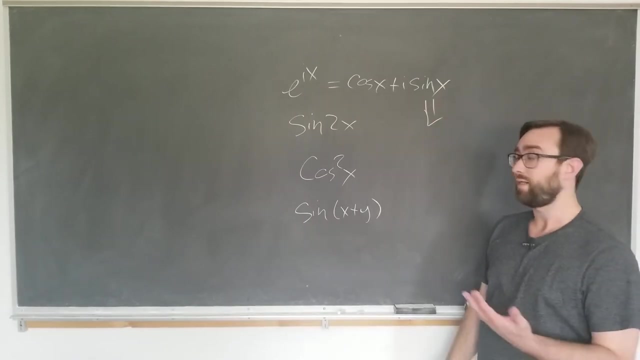 So let's get started. Of course it's going to rely on Euler's identity. e to the ix is equal to cosine x plus i sine x, And you can also show that. this tells you, if you add and subtract it, that cosine x is equal to sine of x, And you can also show that this tells you. 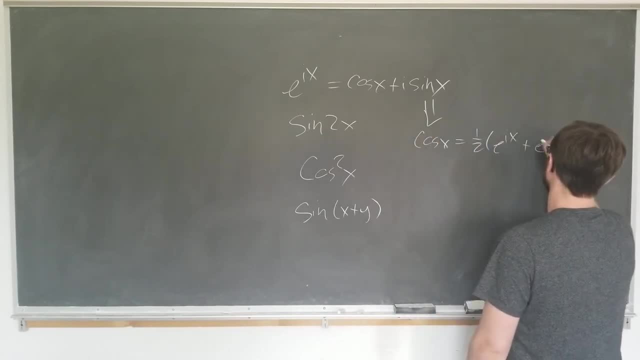 that sine of x is equal to 1 half e to the ix plus e to the minus ix. And sine x is equal to 1 over 2i e to the ix minus e to the minus ix. You do this by adding and subtracting the equations from each. 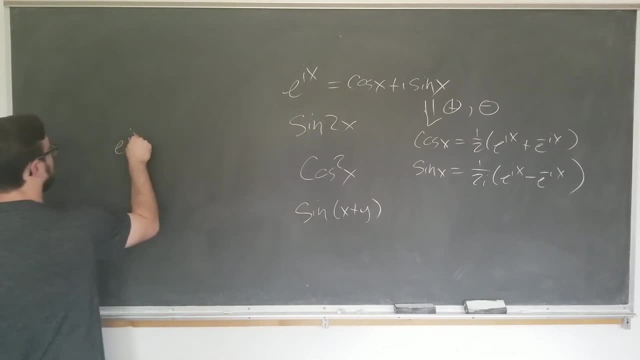 other respectively. So if I want you know, e to the ix plus e to the ix, I would just- I would just evaluate that So that it's equal to twice the cosine. And do the same thing. Take e to the ix and subtract e to the minus ix. from it You'll see that it's equal to 2i sine of 2x using Euler's. 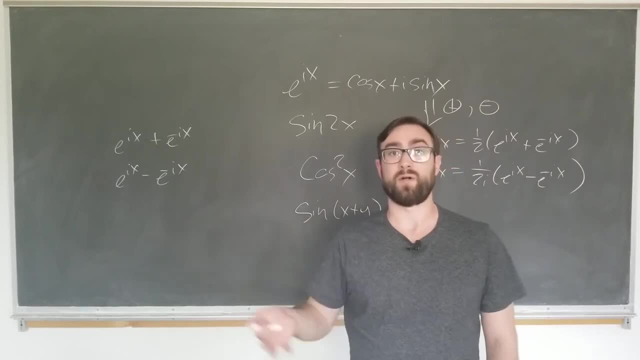 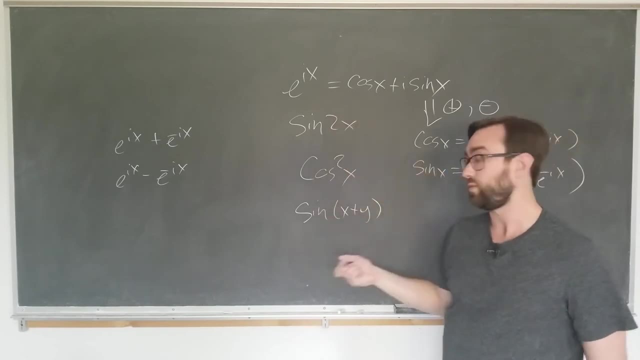 formula Going from there. But that's just review. I assume that you already know how to do that before this video gets started. The new part is to show how to use Euler's formula to evaluate things like this, So let's do that, Okay. 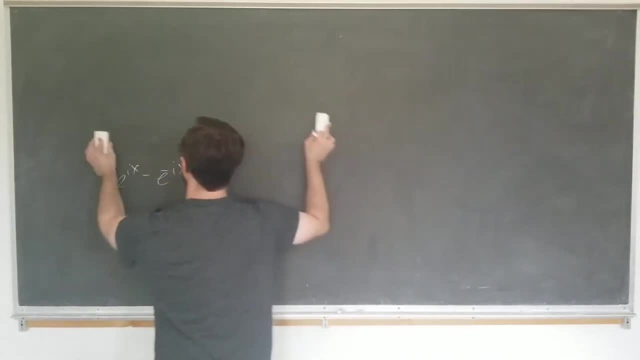 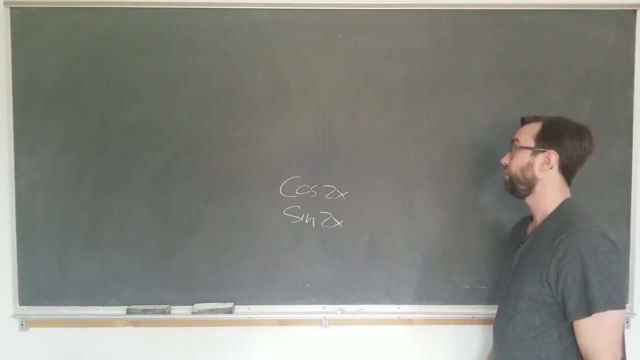 Let's start by it came across cosine 2x or sine 2x on an exam And you didn't remember which formula was which. So we're going to start by considering the complex exponential that this is the real and imaginary part of. So we're going to consider e to the 2i x And we're going to start by considering 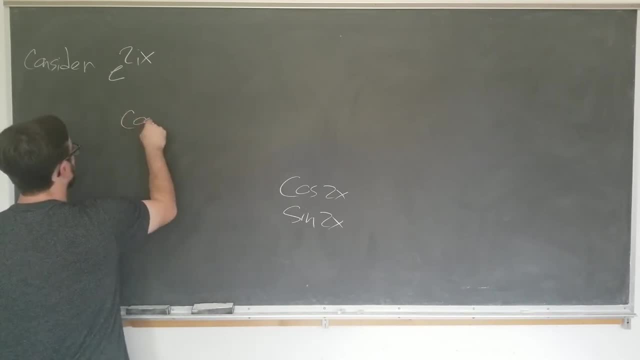 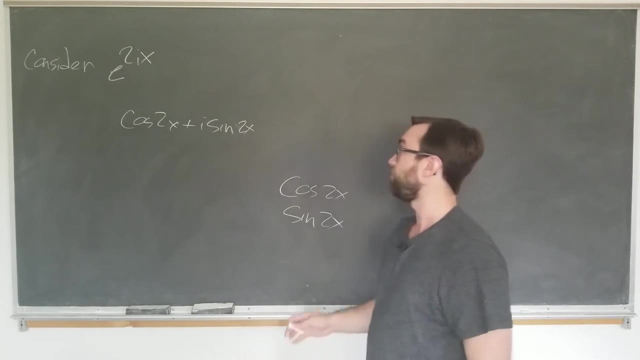 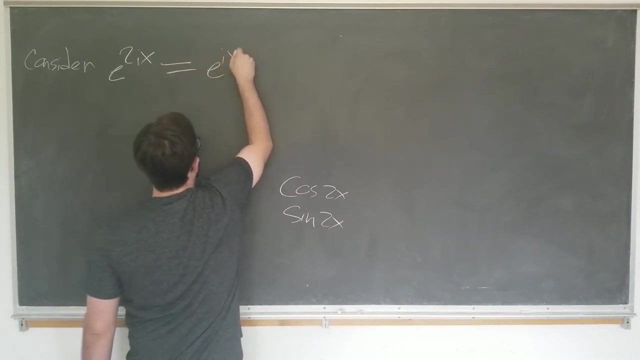 this, And obviously this is just equal to cosine 2x plus i sine 2x. And if we find the real and imaginary parts of this top expression, we'll also find the parts for the bottom expression. So that's all we have to do. By the properties of exponentiation, this is equal to e to the ix squared. 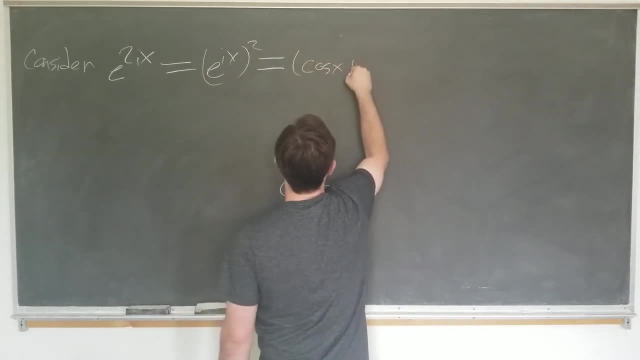 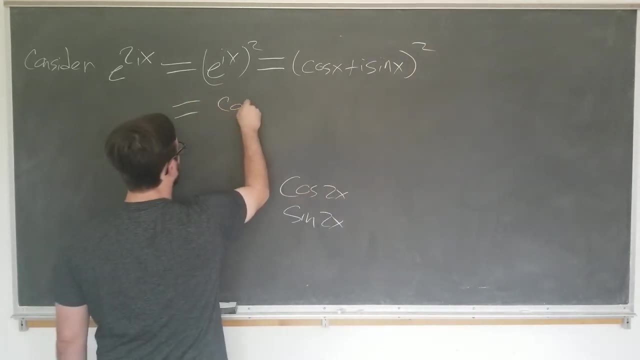 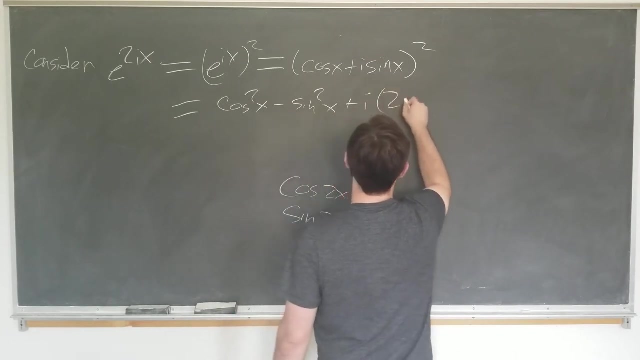 which allows us to use Euler's formula: Square that bad boy. now It's equal to cosine squared x minus sine squared x. plus our complex part, We have 2 sine x cosine x, And there you have it, We're done. So this is actually cosine 2x. This is 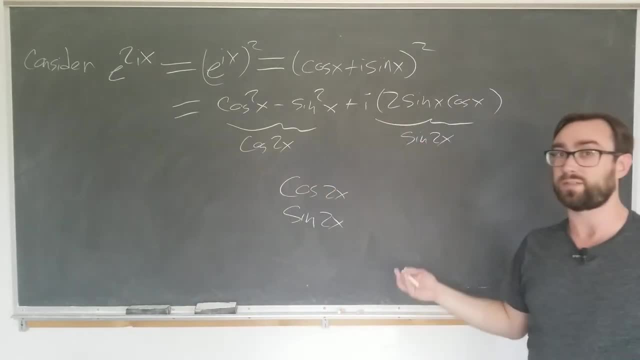 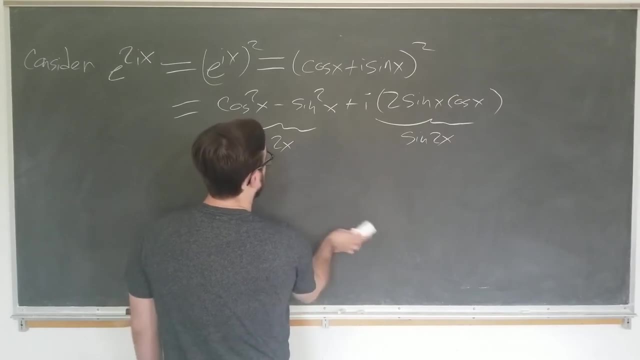 actually sine 2x. I don't think there exists a faster and easier method to derive these equations. If you're going to do it, you're going to have to do it, So let's do it. If you find one, definitely let me know. And, as you might be aware, this is actually just a special case of the. 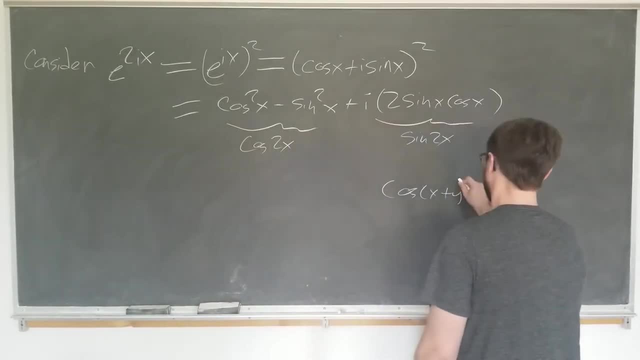 addition formula. You know cosine x plus y and sine x plus y, which also appear on the exam, And we note that it's a special case of cosine x plus x is cosine of 2x here. That's what we derived up here, Just a special case. 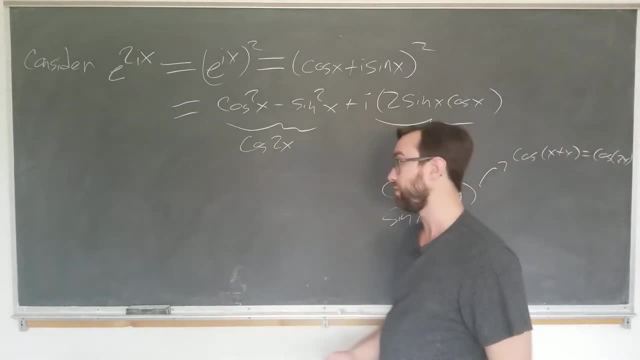 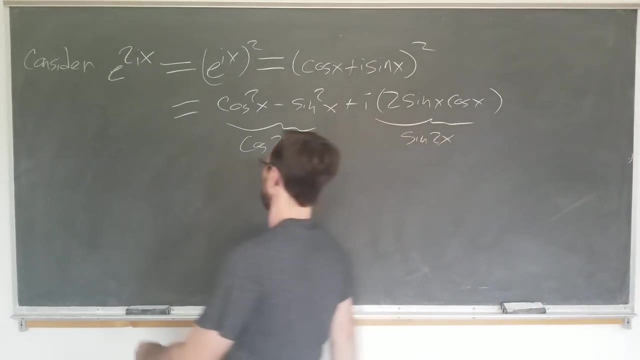 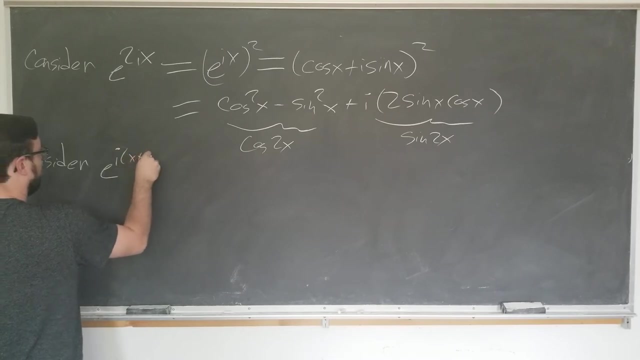 of the addition formula, So we want to derive those as well. Thankfully, they're pretty easy using the same method, Just a bit more abstract. So now we're going to consider e to the ix plus y. Of course, this is going to be cosine x plus y. 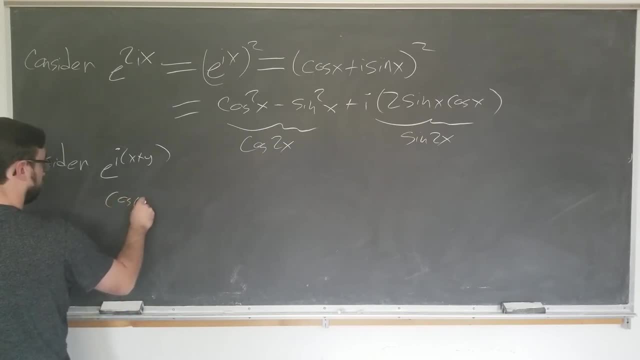 plus i, sine of x plus y. That's why we're considering it, of course, But that's not really part of the derivation- You have to keep this in your head in advance- which you would in an exam anyways. It's equal to e to the. 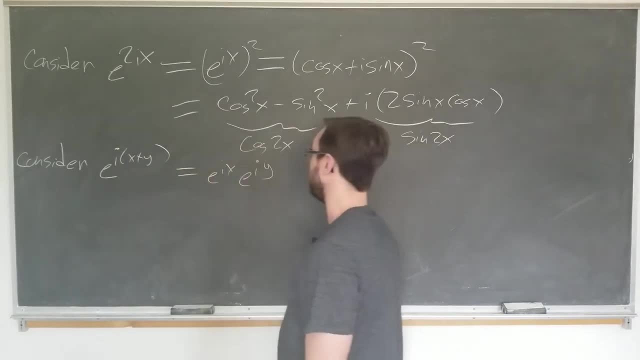 ix, e to the iy by the properties of exponentiation. Note: it's the same above if x is equal to y. So that's how this generalizes, Using it twice here. Euler's formula that is This is cosine x plus i sine x. 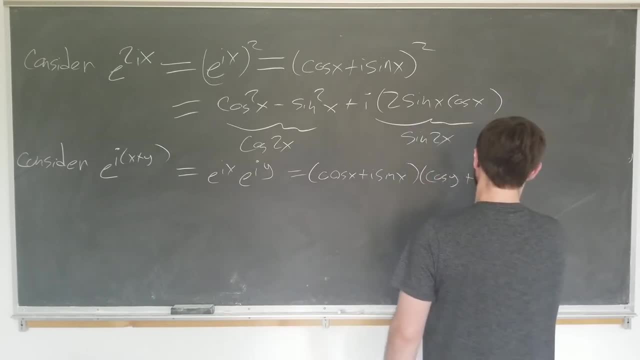 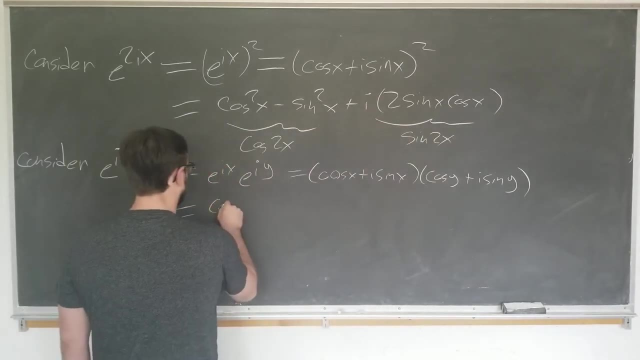 and cosine y plus i sine x. So that's how this generalizes, Using it twice here. Euler's formula, that is This, is cosine x plus i sine x and cosine y plus i sine y. Using the FOIL method, this is just equal to cosine x, cosine y plus imaginary term. 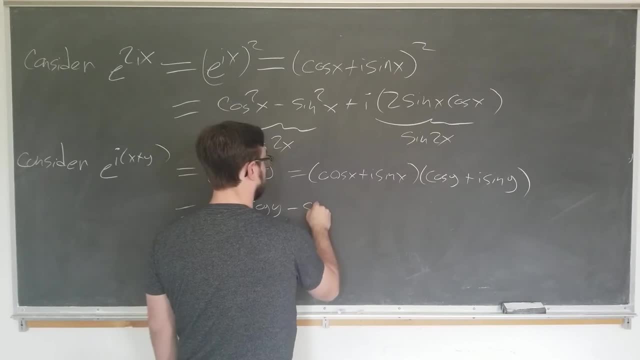 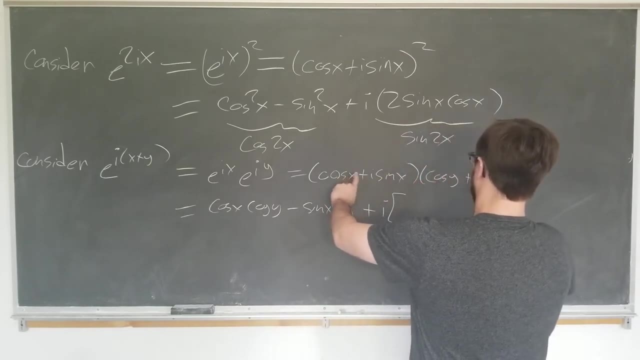 the imaginary term, real term, minus sine x, sine y. Now we have the imaginary term. We did that, now we do this, Now we do our��은 반. So we get the positive gentrion here. theospheric term sine of x and sin y and cosine y. 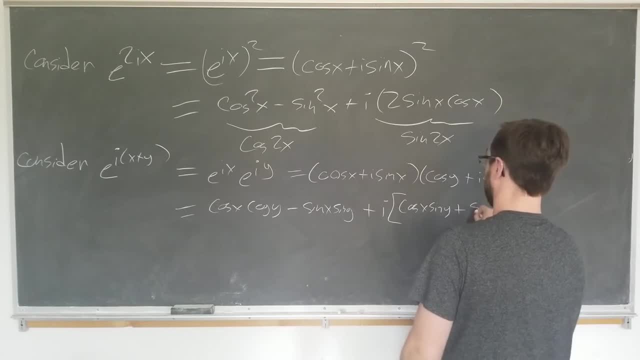 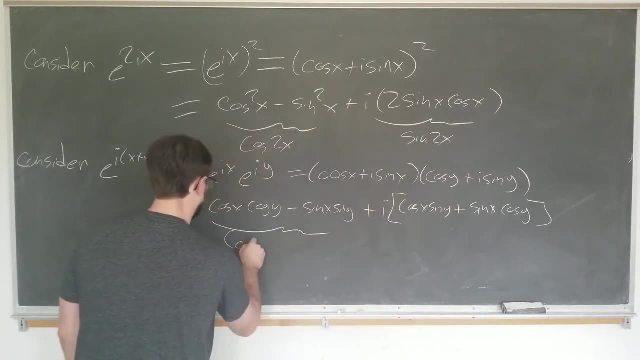 So we have sin x and sin y and the imaginary term there. Now we have 2 daqui And now we get cosine x and sin y. This is cosine x sine y, And we'll use that here and adjust it: this plus sine x, cosine y, and we're done, since this is just cosine x plus y and 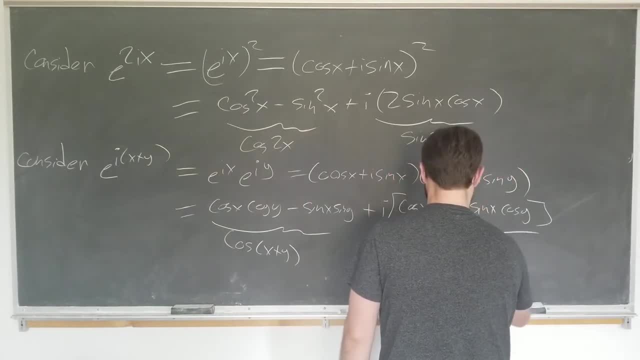 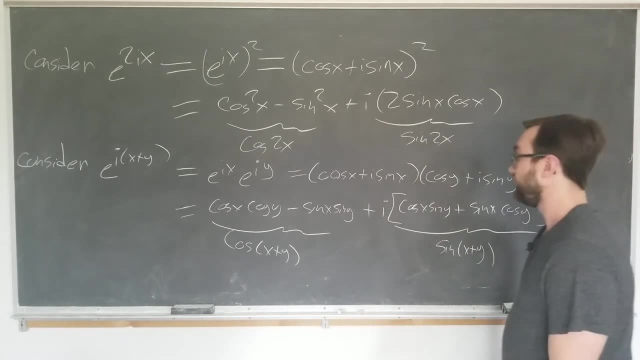 this is just sine of x plus y. feel free to check it. I hope I got it right. if not, it's pretty much what you do here, so you can definitely prove me wrong in the comments. okay, so this is about the only identity that you can derive by. 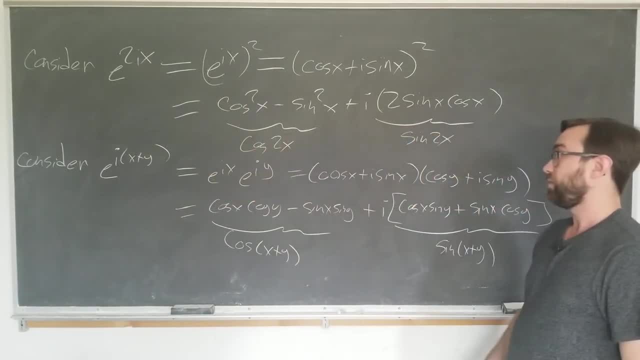 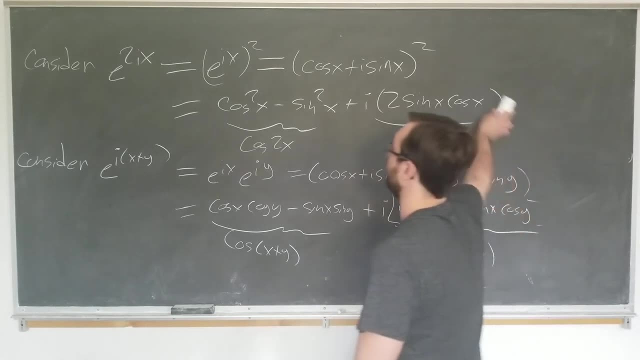 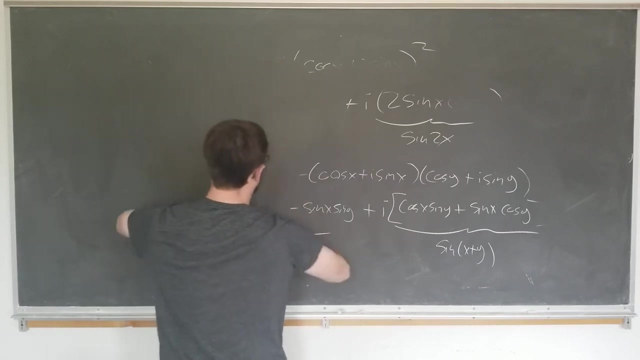 considering the complex exponential itself. since these are the only identities that are linear in the arguments, there are many other identities that you need as well that are not linear, so let's discuss how you would derive those. as you can probably guess, we're going to use the second. 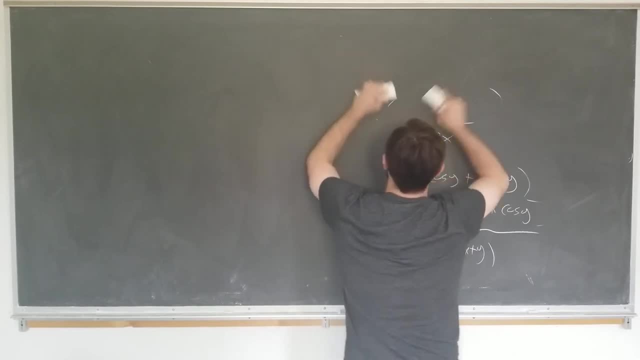 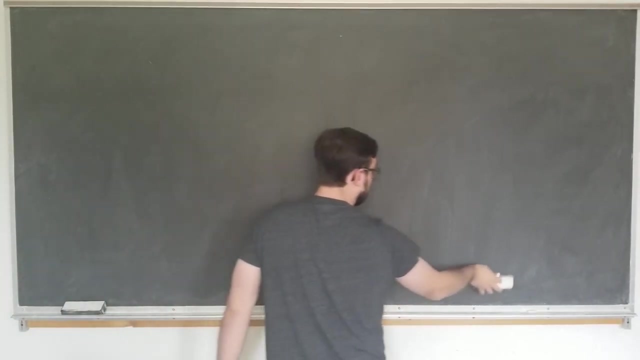 method where we write out sine and cosine directly in terms of the complex exponentials, with the appropriate factors of 2 and I, of course, and go from there. as you've seen already, these derivations are much easier than other derivations you've seen because we can use the properties of exponentials, whereas with 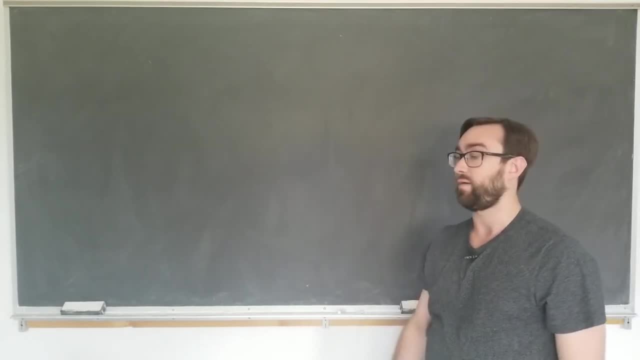 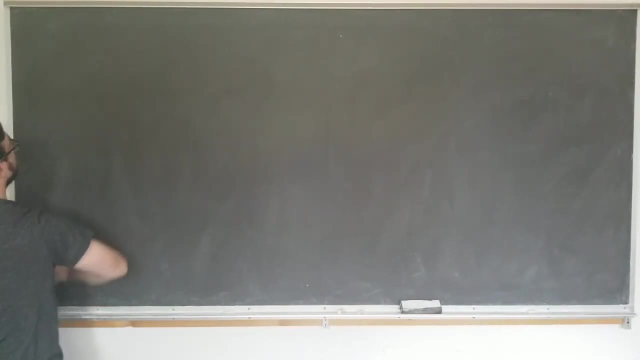 other non-complex identities, we'd have to rely on other trigonometric identities to derive ones that we're trying to discuss. alright, so now we want to evaluate cosine squared x. why? well, what if we have the integral of cosine squared x and the exam? for some reason, you had to integrate it. well, it'll be much easier to use the identity which 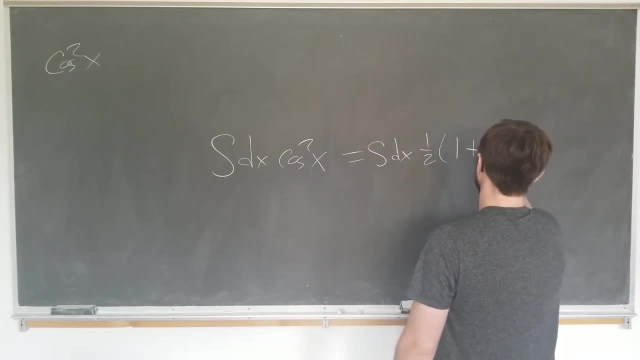 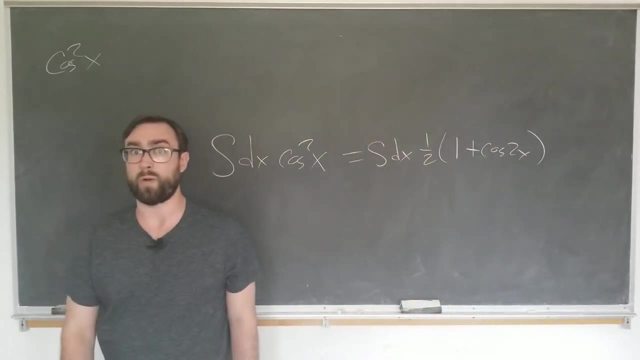 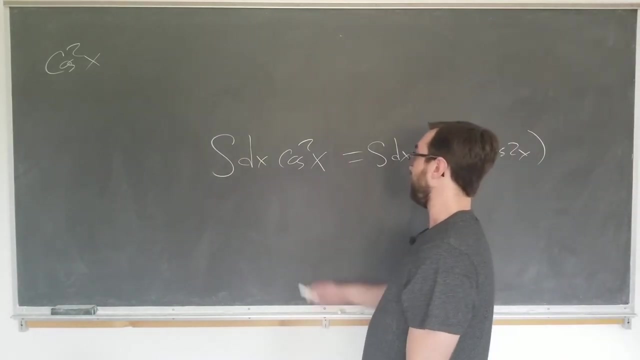 we're going to show one half of one plus cosine two x and integrate it directly. so, yeah, this is what we want to show. also a similar identity for the sine function, which we'll derive shortly, but this is the primary reason that I had to use this identity, though of course, there are many. 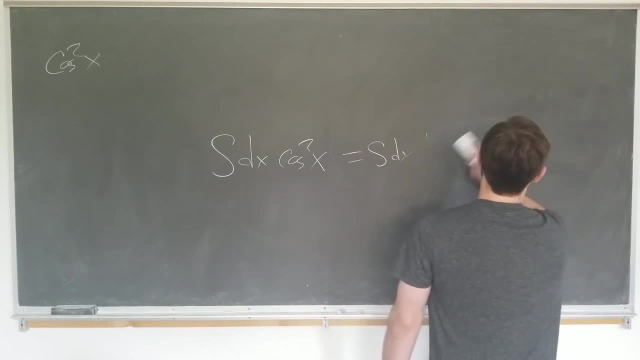 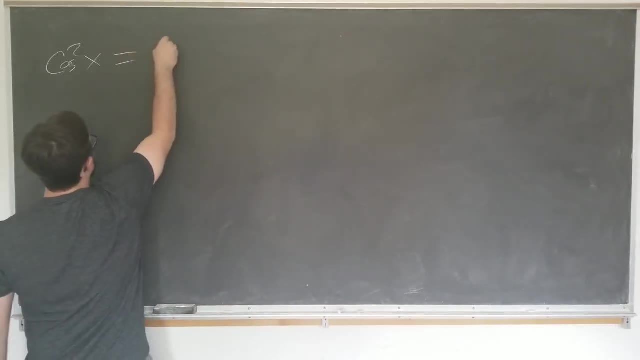 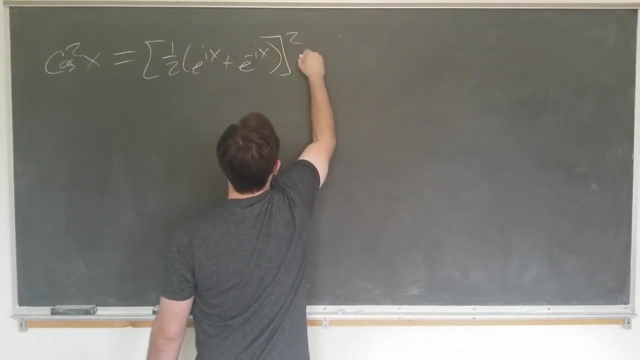 other reasons that you might have to use it as well. all right, so we're going to write this as one half: e to the i x plus, e to the minus i x squared. we're going to get two factors of one half, which we're not going to combine into one fourth for reasons that you're going to see. 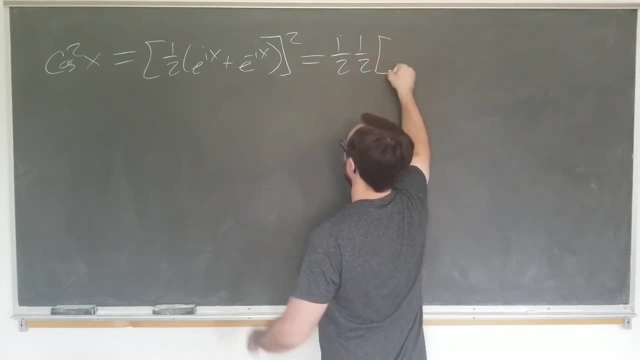 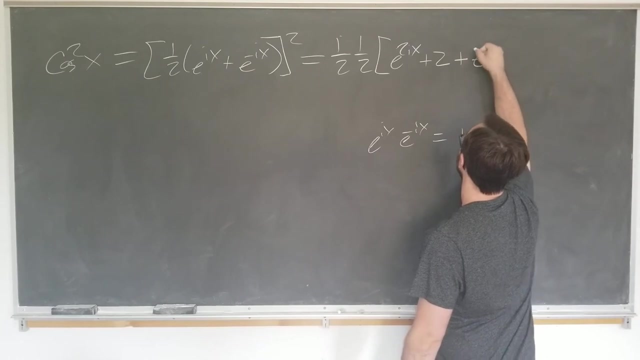 momentarily using the foil method, we're going to have e to the two i x and plus two times the middle term, which is just two, since e to the i x, e to the minus i x is equal to one, of course, plus e to the minus two i x, which we're going to simplify now as follows: 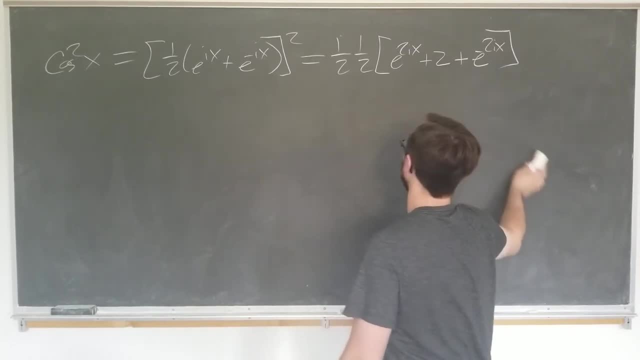 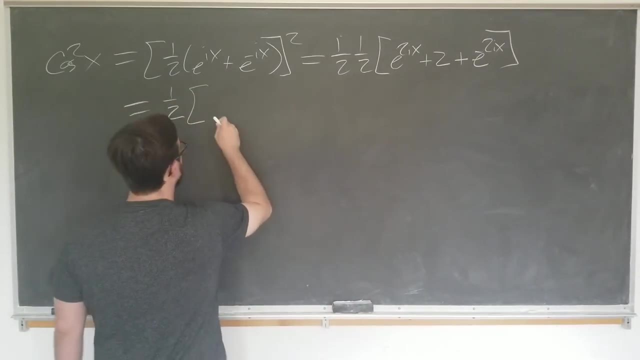 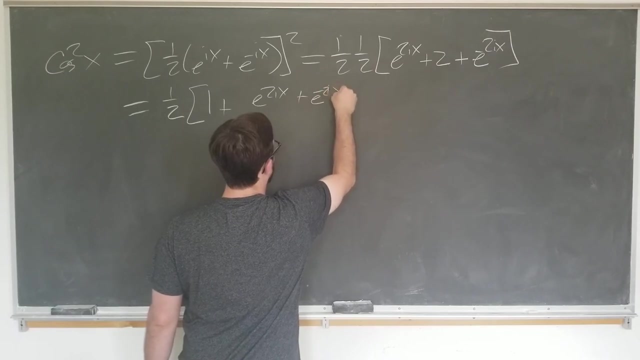 we're going to take one of the one halves and distribute it through, so it becomes one half. we're going to put the constant up front. we have one plus e to the two, i x plus e to the minus two i x divided by two, and you can see where we're going here now. this last term is just the cosine of two x. 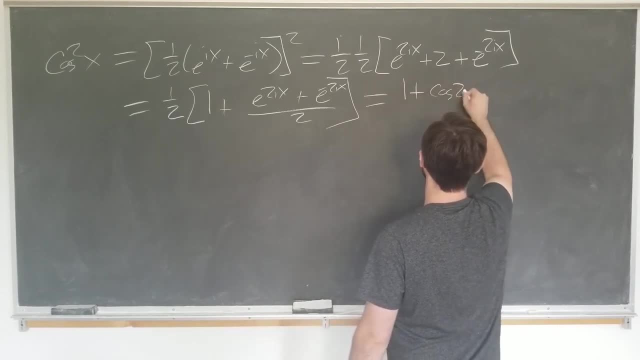 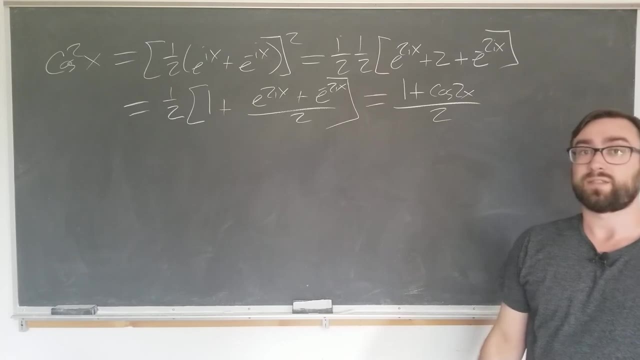 so it becomes one plus cosine, two x over two. exactly as I told you. it was excellent, it's great, but because we did not consider the complex exponential at the beginning, we have to do a similar derivation twice for the sine function. so let's, let's do that now. 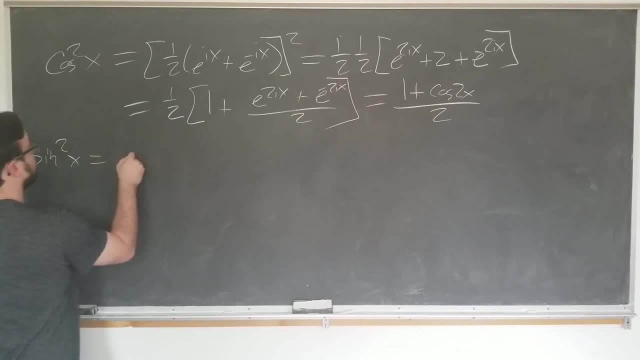 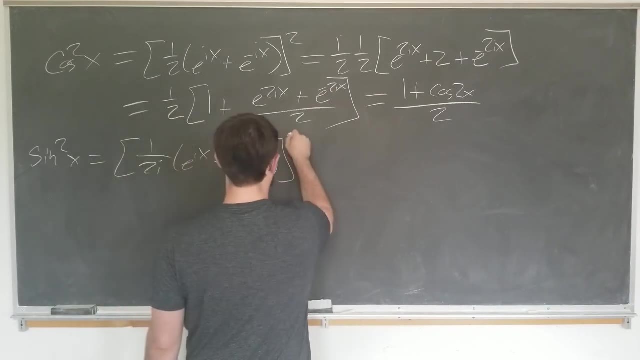 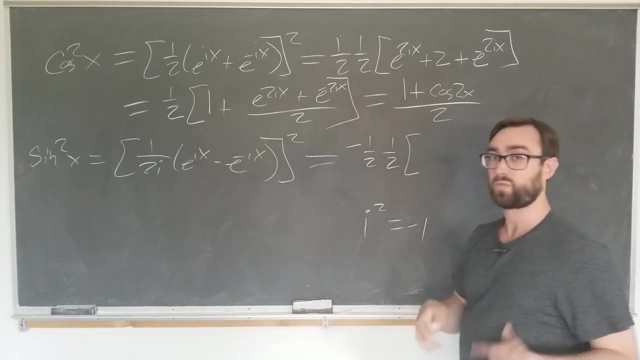 sine squared of x is equal to one over two i e to the i x. minus e to the minus i x, everything's squared. so i squared is equal to minus one, of course. so we're going to get minus one quarter, which we'll write like this: minus one half times one half. and now distributing, squaring rather, 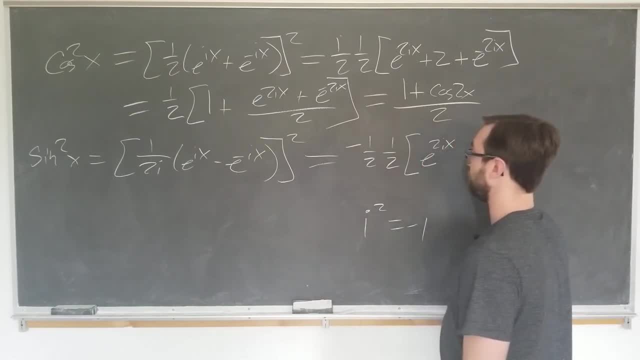 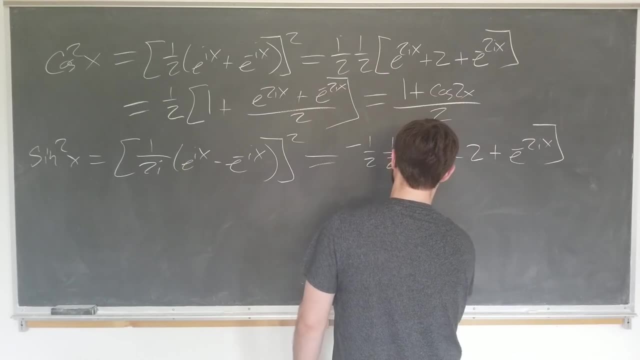 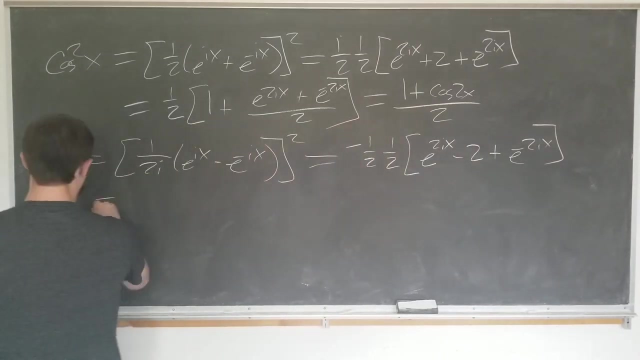 so we have e to the two i x. again we have minus two plus e to the minus two, i x. and now we're going to take the minus a half distributed through and keep the plus a half up front, one half, and we're going to put the constant up front so it becomes one. one half times two is one. 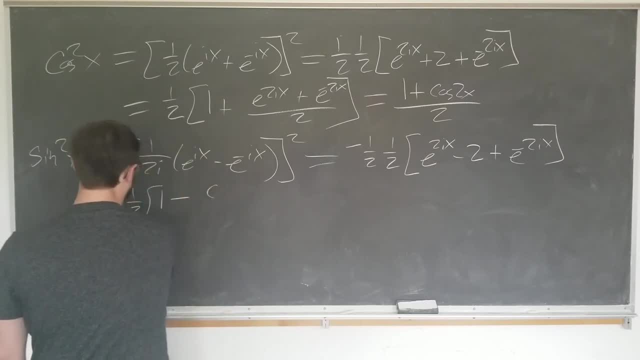 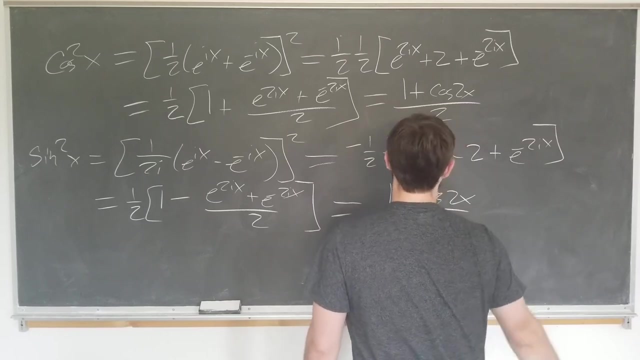 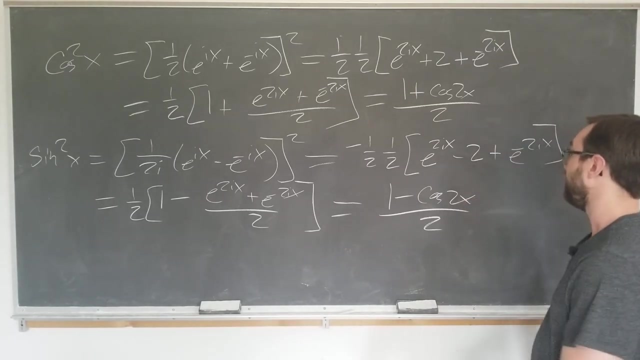 of course, and that's going to be minus, not cosine, yet not cosine yet. e to the two, i x plus e to the x over two, which is just simply one minus cosine, two x over two. incidentally, there is another way to recall these as well: i always check it for the value at zero. i know that if i, if i square, 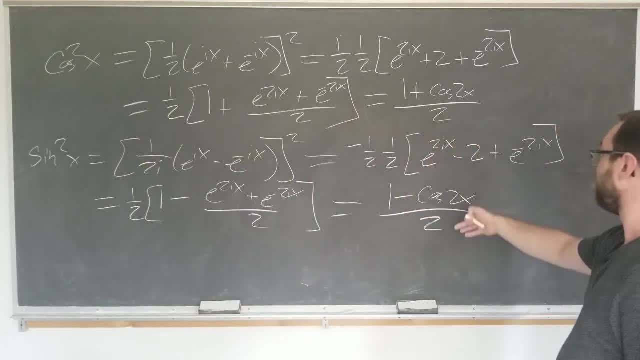 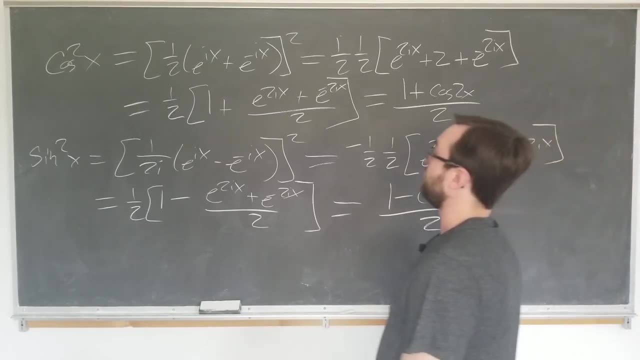 a cosine or a sine. it's going to involve one and cosine two, x and two. so if i want to know which one is which i plug in the limits, since cosine squared of zero should be one and cosine two x is one, and if i plug zero into here, i get one plus cosine zero is one over two. one plus one. 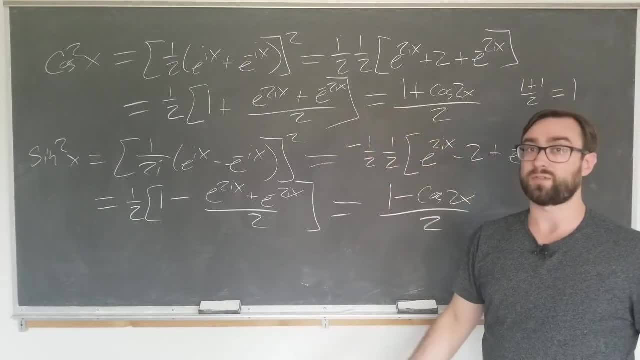 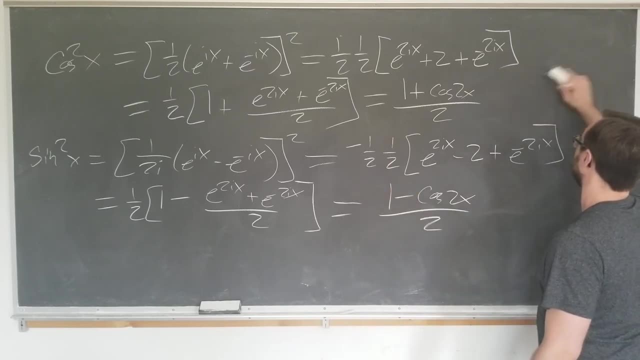 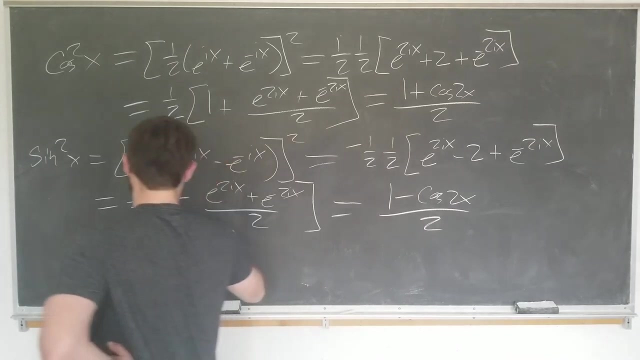 equals one, of course, so i know that this one has to be cosine of two x and the other one, excuse me, has to be sine squared of x. so yeah, that's how you can do that, and it doesn't have to stop here. you can apply the same principles to derive many other identities, like sine squared. 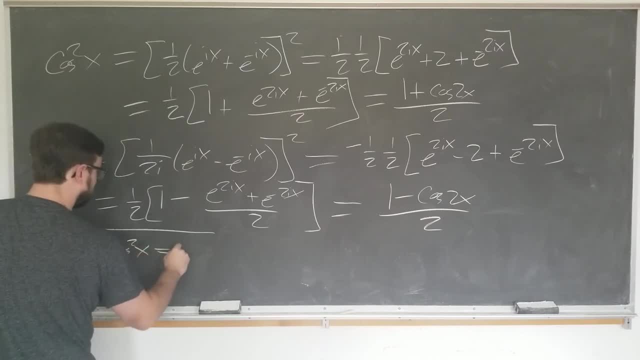 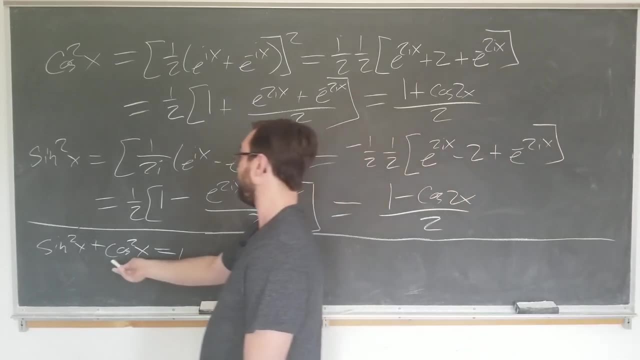 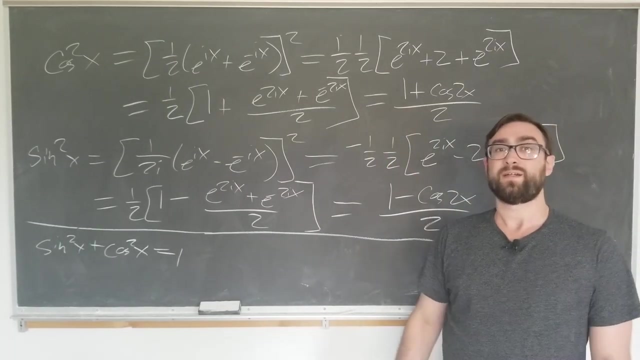 of x plus cosine. squared x equals to one. it can be derived in much the similar fashion that we have done here. you just put the euler formula versions of sine and cosine. i don't really feel that this identity fat, fat the topic of the video, since i can always remember this one. i think everyone remembers this. 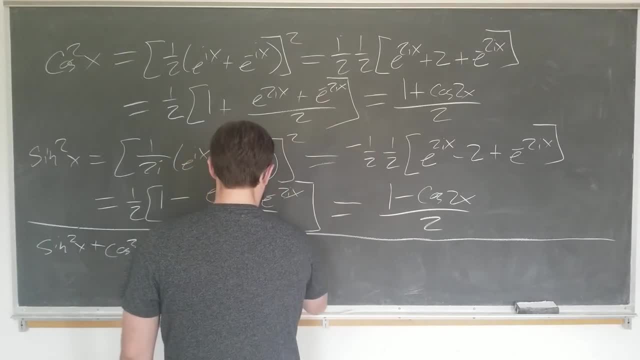 one. there are also things like, if you wanted to know about sine of pi over two minus x, for example, is it true that sin squared x is one of the properties that we have in the problem of sine squared x and sin squared x is one of the properties of the problem of sine squared x? as we've seen in the equation of sine squared x, 2 minus sine squared x into sine squared x is a integral of sine squared x. you can call: fit that into that. so anyway, this is just a formula. you just can very easily derive the difference. but it's the 250 points for each element and that's why i wanted this.